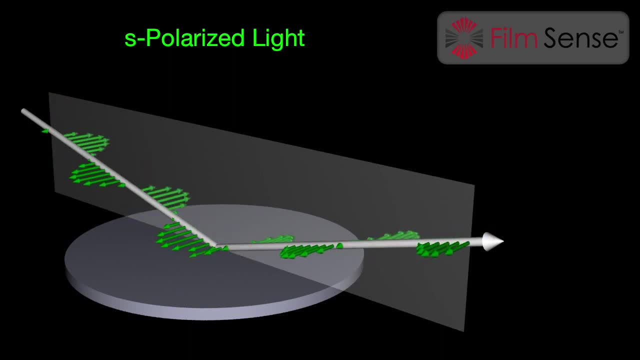 perpendicular to the plane of incidence is called s-polarized light. The enabling principle of ellipsometry is that p- and s-polarized light reflect differently. Ellipsometry measures the complex reflectivity ratio of p- and s-polarized light, and typically 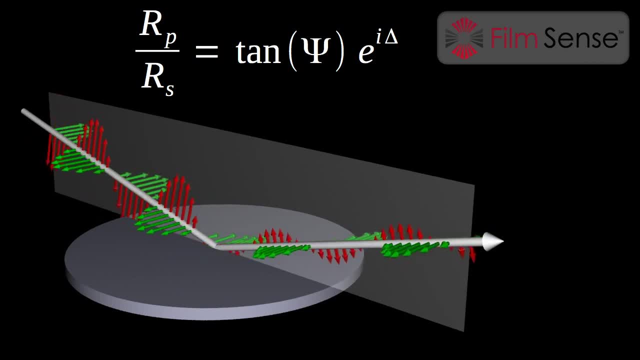 reports the results in terms of the ellipsometric psi and delta parameters. Tan psi is the magnitude of the ratio and delta is the phase difference between the p- and s-reflected light. To measure the ellipsometric parameters, an ellipsometer system must set the polarization. 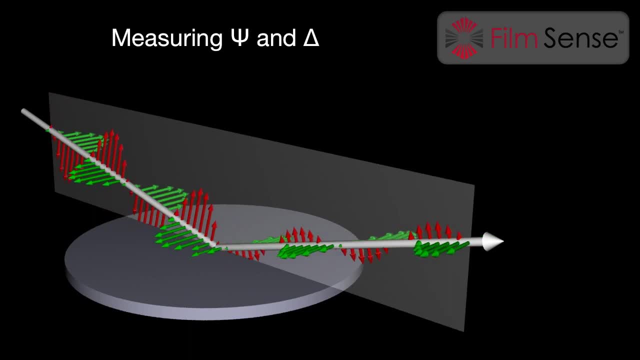 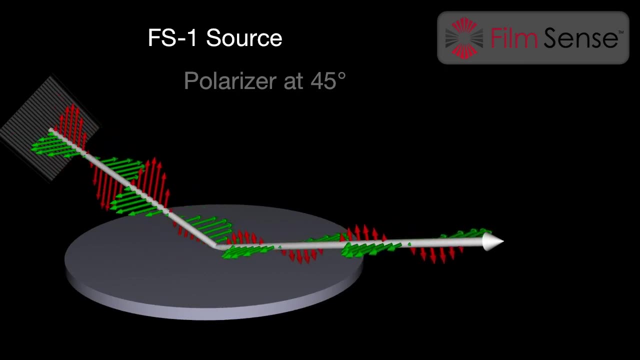 state of the incident beam and detect the polarization state of the reflected beam. In the FilmSense FS-1 ellipsometer, a polarizer in the source unit sets the incident beam to a linear polarization state, rotated 45 degrees from the plane of incidence. 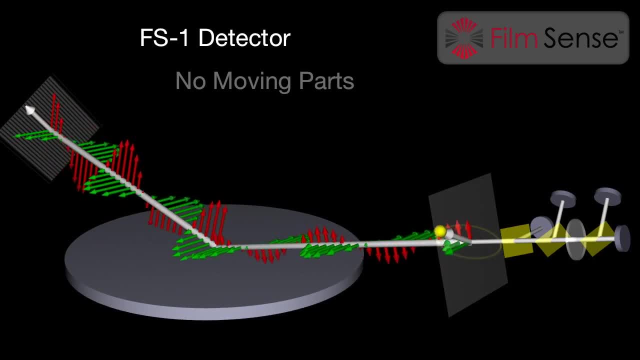 The FilmSense FS-1 detector unit contains a proprietary combination of b- and s-polarized light, The beam splitters and optics which split the beam into multiple beams and detectors, each sensitive to a different polarization component of the incoming beam. 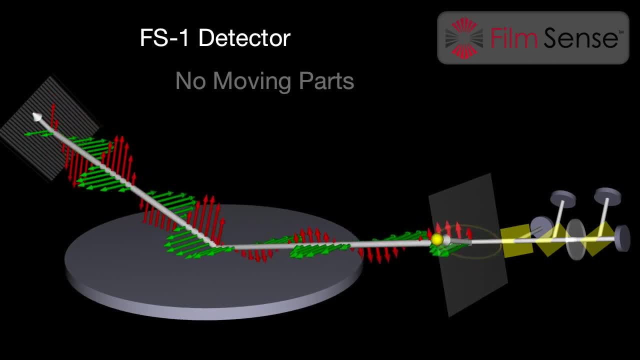 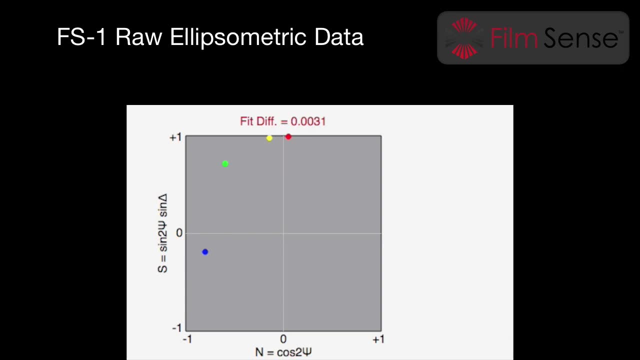 This provides fast, accurate and reliable measurements of the ellipsometric parameters without any moving parts. The FS-1 software plots the measured ellipsometric data as colored points on a 2D plane. The four colors correspond to the four FS-1 measurement wavelengths. 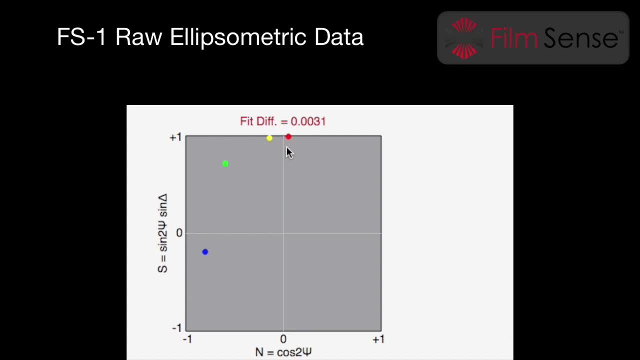 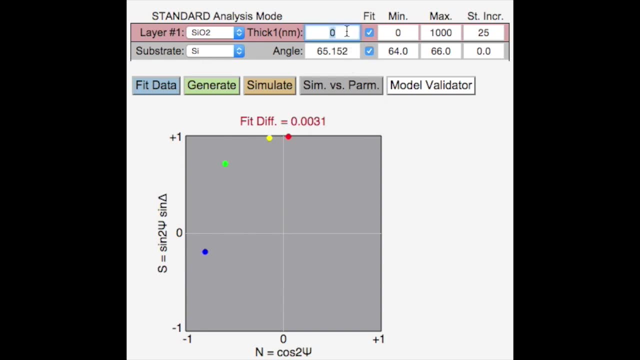 To determine film thickness or optical constancy, it is necessary to measure the ellipsometric data set. An optical model is defined corresponding to the structure of the sample Model. parameters such as film thickness are specified. The optical model can generate an ellipsometric data set which is shown on the plot as open. 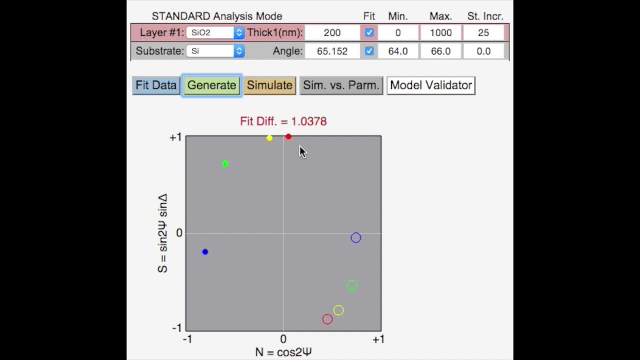 circles At this specified thickness. the model generated data does not fit the measured data very well as quantified by the large fit difference value. When the fit data button is clicked, the software is able to calculate the measured fit difference. automatically searches for the parameter values which minimize the difference between the measured 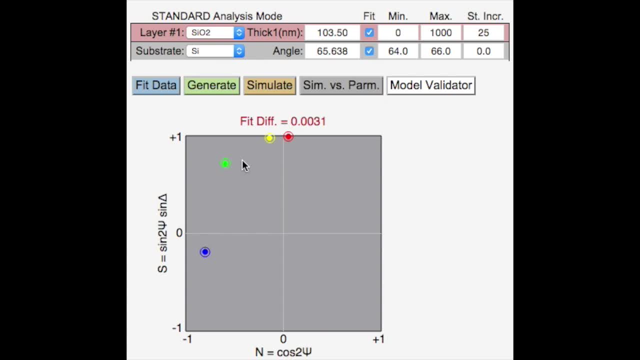 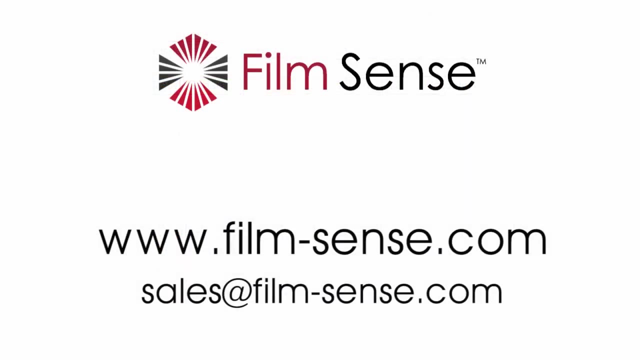 and model generated ellipsometric data sets For a good fit. four bullseyes appear in the plot. the fit diff value is low and sample parameters such as film thickness are determined with excellent accuracy. Thanks for watching this introductory video on ellipsometry and polarized